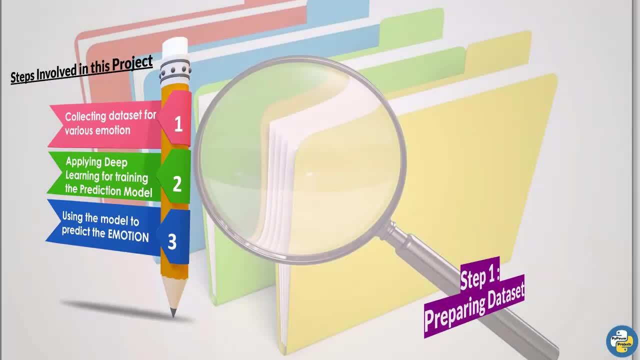 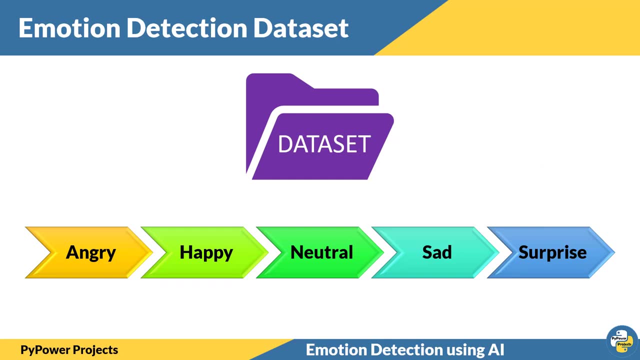 the person's face. Step one: preparing data set. In this data set, we have curated total five classes that are total five emotions: angry, happy, neutral, sad and surprise. These five types of emotion can be detected based upon our data set. 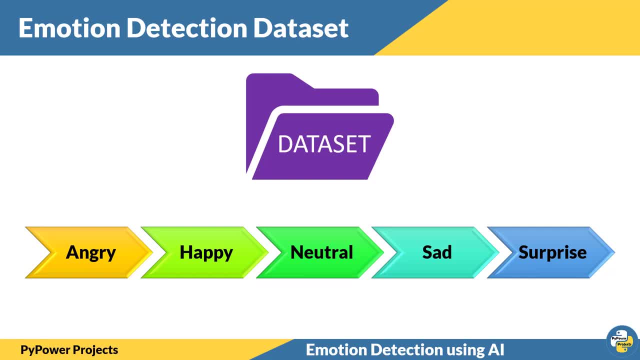 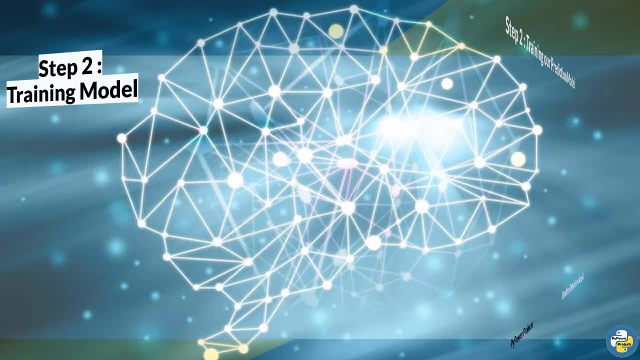 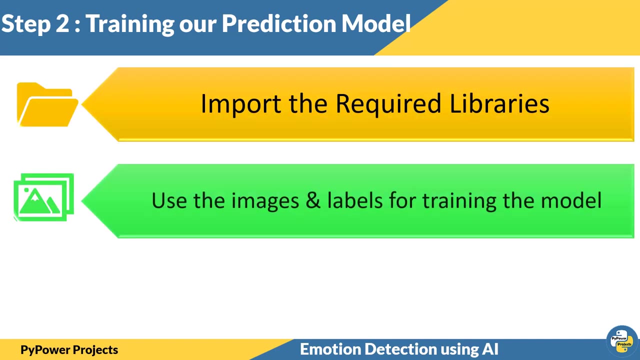 You can increase the number of emotions by collecting the data set of that particular emotion while training the model. Now comes the step to training the model. In this, again, there are total three steps. First, we will import the required libraries. Second, we will use the images and labels for training the model. and finally, using Keras. 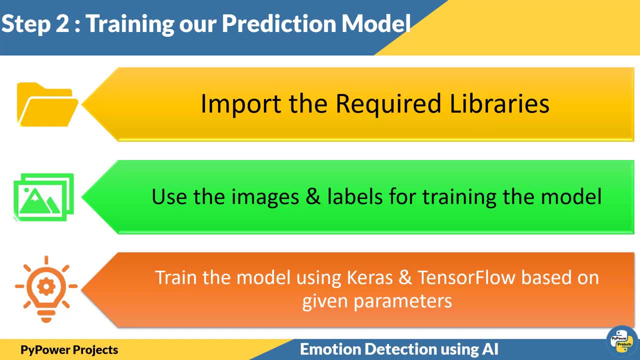 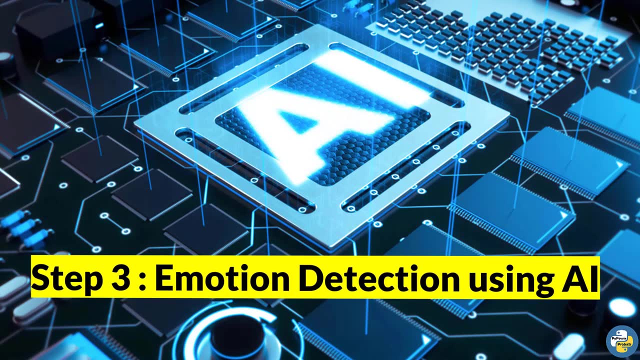 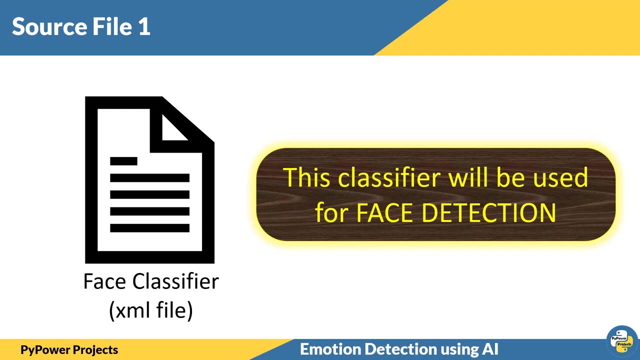 and tensorflow. based upon given parameters, we will train the model. Last but not the least, step number three: emotion detection using AI. Now how this emotion is detected. for that we will require total three source files. that is, three files will be required for overall execution of this project. 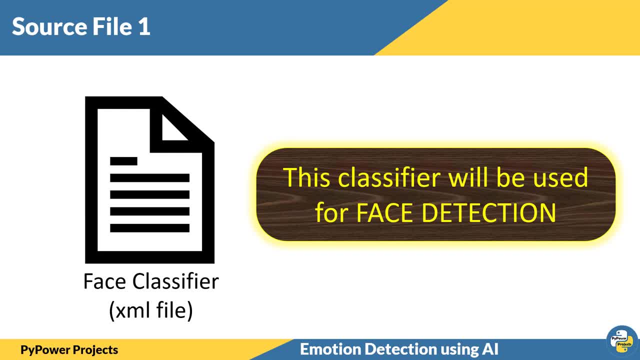 First is the face classifier. So what this face classifier will do? it will detect that, whether the input frame- that is, in the video, Whether there is any face or not, Because once the face is detected, then only we will able to detect the emotion. 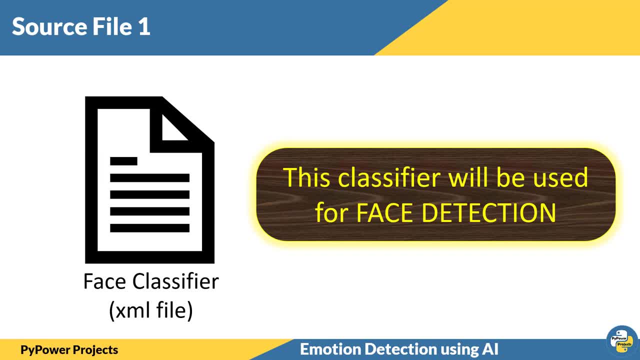 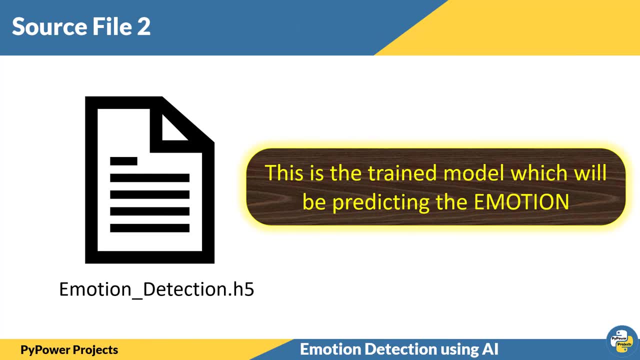 So, first of all, this face classifier will detect the face and further in the second source file there is emotion detection dot h5.. So what is this h5 extension? This h5 extension is commonly used for the trained model. The model which we have trained will be stored as emotion detection. 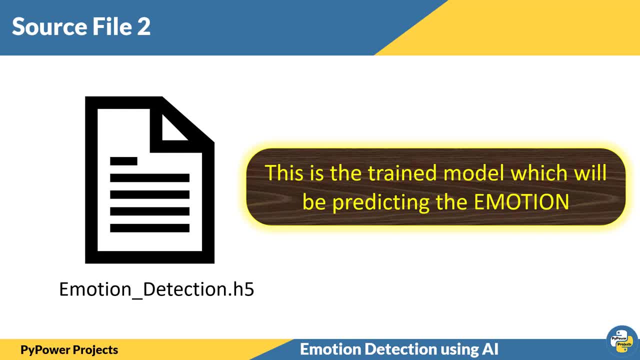 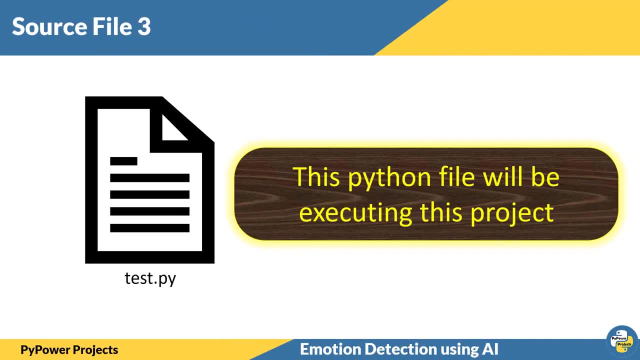 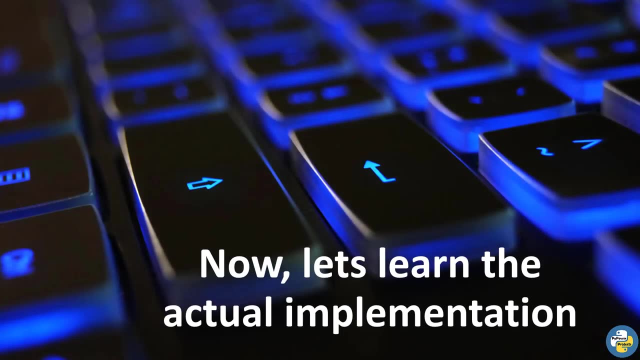 H5. And we will be using this trained model for predicting the emotion. The third source file is test dot py. This is the python file we will be using for executing this project. So now let's learn the actual implementation of the code. 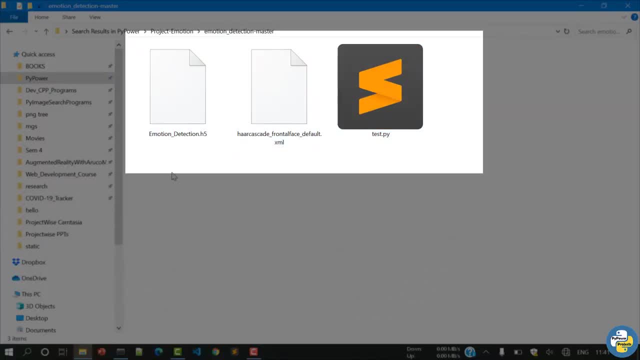 Yes, here you can see that here in the folder there are total three files: emotion detection H5.. This is the Keras trained model. Second is the exception. This is the xml file that is the face classifier. and third is the test dot py. 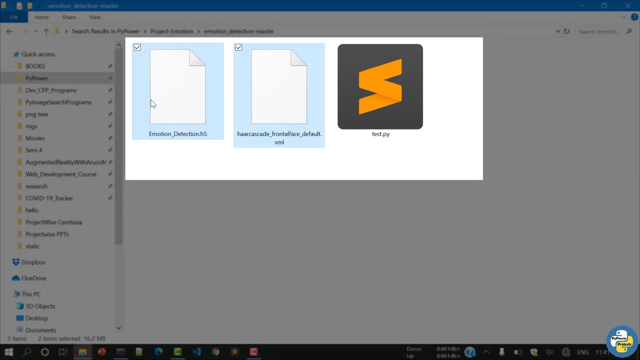 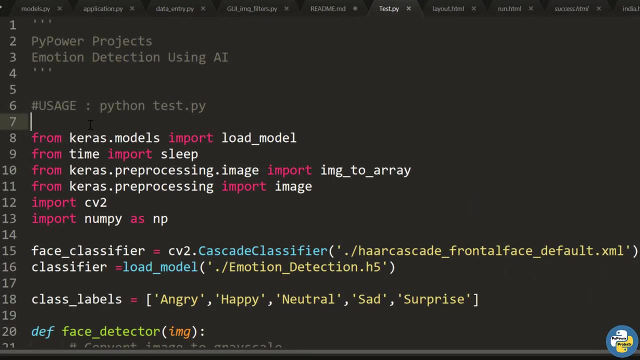 This source file will take use of this both file, that is, face detection and emotion detection, and will process the whole project. Before going in more detail, first you will see how to use this file. So for that you have to open your command prompt or terminal, and in that you have to. 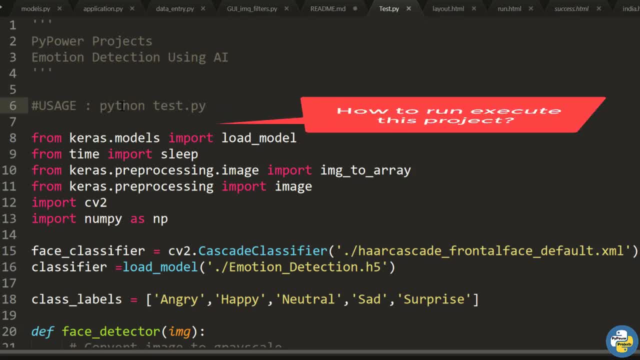 type: python test dot py. The file name is test dot py. So you have to open the terminal and write this command: python test dot py. So you have to open the terminal and write this command: python test dot py. It will execute this file, it will run this file and do the emotion detection. 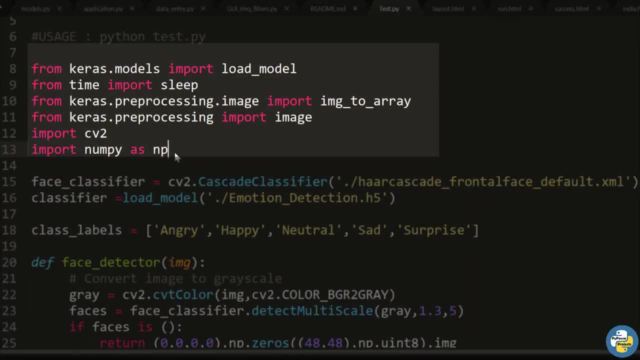 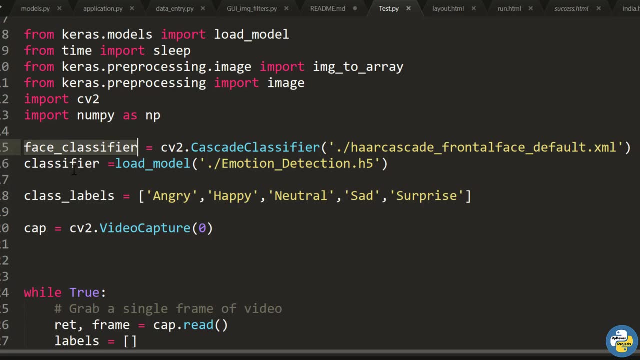 Here we have imported the required libraries, the Keras open CV and the numpy. So now, first of all, we have initialized the face classifier and secondly, the emotion classifier. The face classifier is the xml file which will detect the face from the input frame, and second is the model file which will be predicting the emotion based on the particular 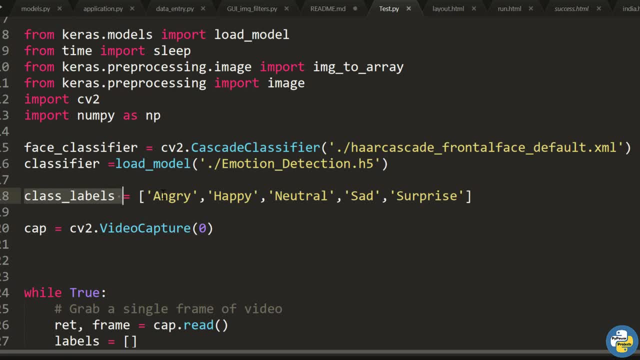 face. These are the class labels. here we have trained our model on these five classes- that is angry, happy, neutral, sad and surprise. So here we have prepared a list of these particular classes. If you're training your model on some different classes or different number of classes, then 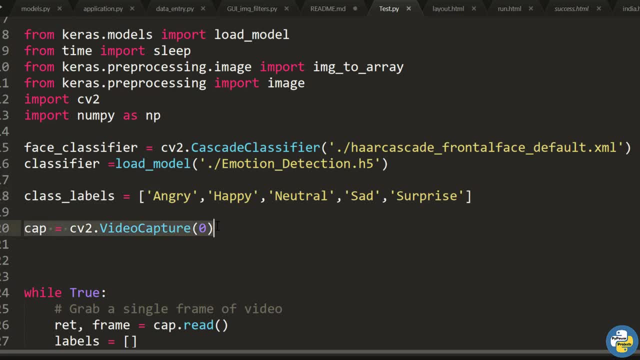 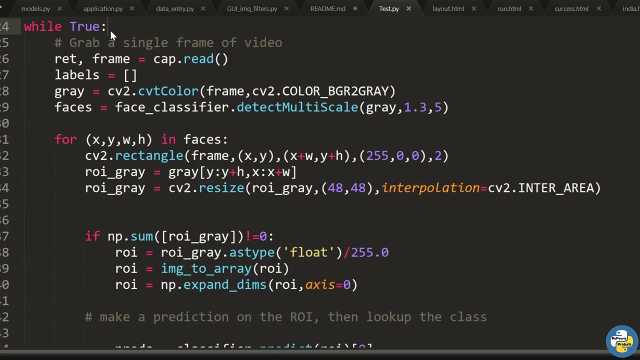 you can change the list as per your requirement. Here we are capturing the video frame from the webcam. Here the video capture takes the argument. if zero is passed as the argument, it will by default access the webcam. Now comes the actual implementation. While true file, true means this is an infinite loop and until you don't stop the execution. 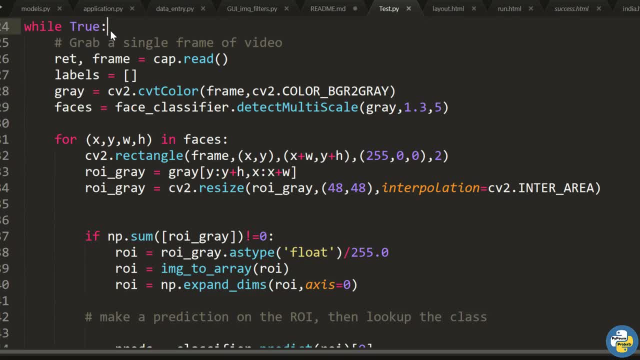 this will continue: the prediction of the emotion. This loop will run forever. So, first of all, we will grab a single frame of the video from the capture object and after that we will convert it into grayscale. After that we will pass that grayscale image into the face classifier. 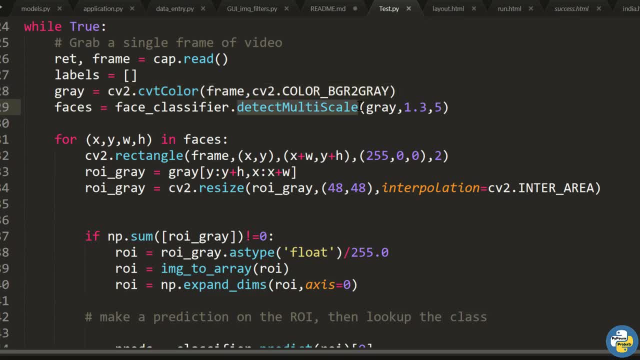 This detect multi scale method will detect the face from that particular image frame in the data. Data will be stored in this variable faces. This will return four variables: X, Y, W and H. These are the coordinates of the face. We will draw a blue rectangle which will be boundering the face so that we will able to 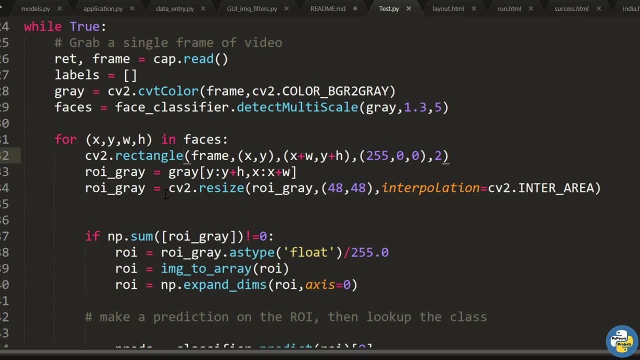 see that if the face is detected and the location is this, we will resize it to 48 cross 48.. So why 48 cross 48? we have to resize because the model which we have trained is on the architecture, mobile net, And in mobile net architecture we have to give the input image in this particular dimensions. 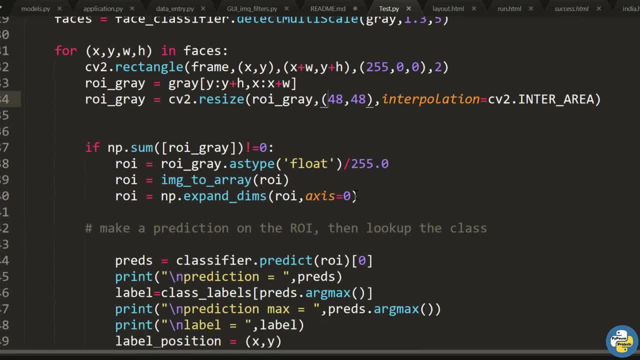 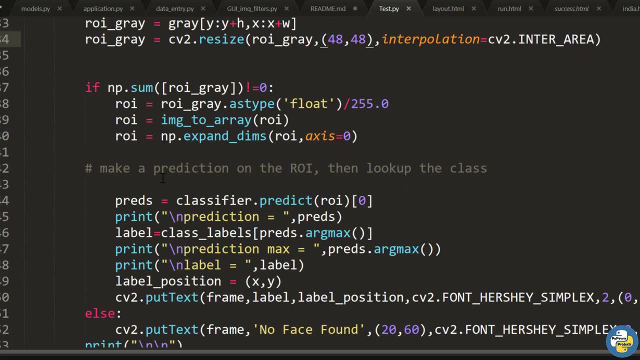 only So we are resizing it to 48, cross 48. After that we are converting the image into the array. and after converting the image into the array, Now we will predict. classifier dot. predict method will predict the probability of each and every particular class here. 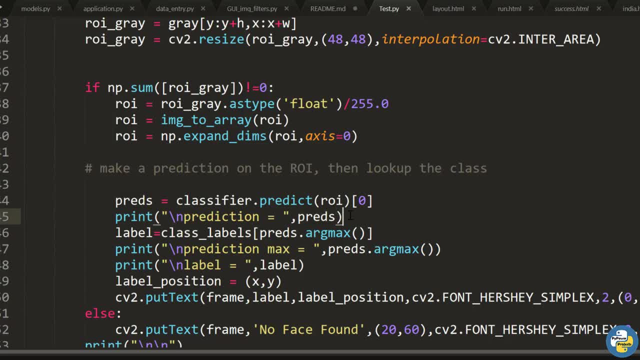 If you print this print That is, Then it will return an array in which there will be probability and we have to choose the maximum probability, that is, which is the maximum possible emotion from this particular image frame. So pretz dot arcmax function will return the index of the maximum probability and we will 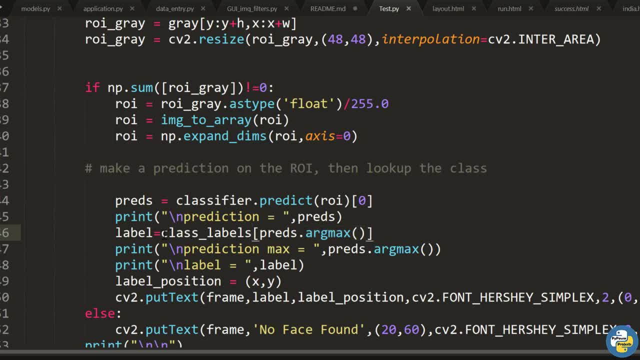 access the name of the class label by this way: class label and in that the index number and after that the label will be Printed in the maximum probability will be printed. this is for only demonstration purpose. it is not required exactly here. So the core part is only this much. 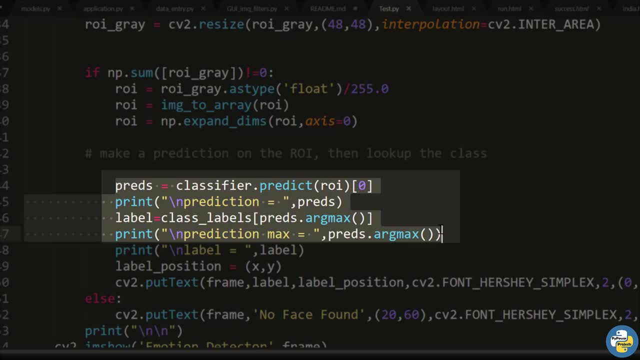 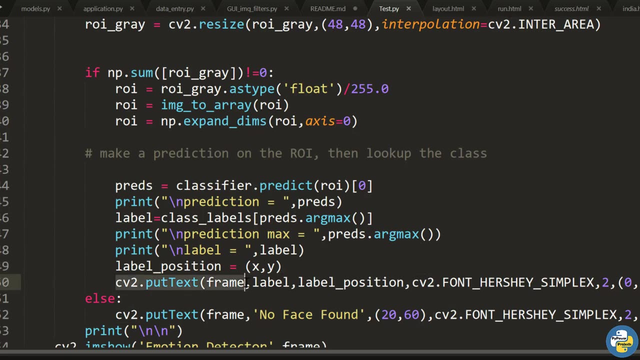 So only these three to four lines are responsible for whole prediction task. After the prediction is done, we will assign the label and we'll put the text on the face that, yes, this is the face and this is the particular emotion that the present input frame is having. 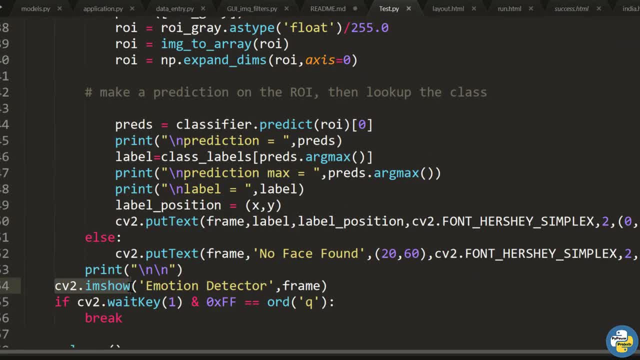 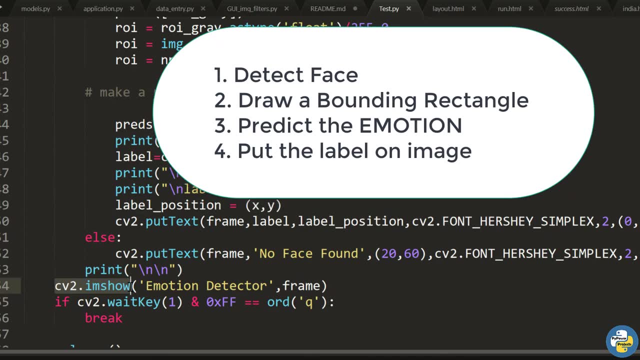 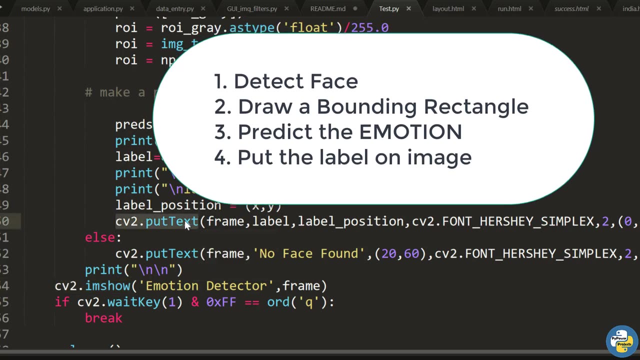 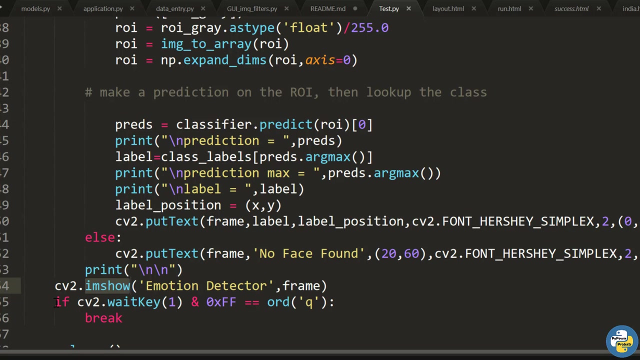 Here, cv2.imshow function will show the output of the emotion detection program and each and every step which we have done for the face detection which will draw a blue rectangle, and after that the emotion which will be printed on that particular box. this whole output will be shown by cv2.imshow function and this is the exit condition, that how you have to close. 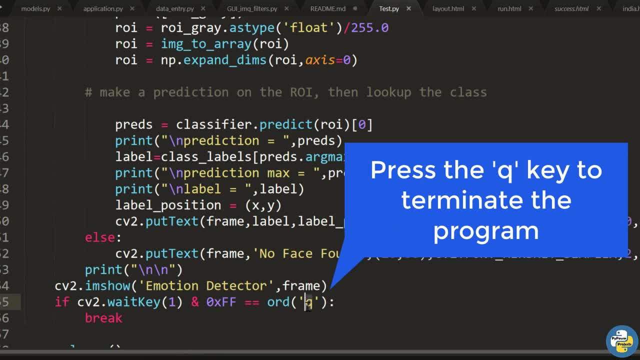 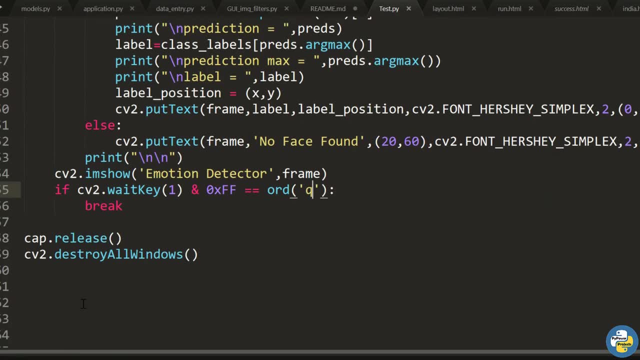 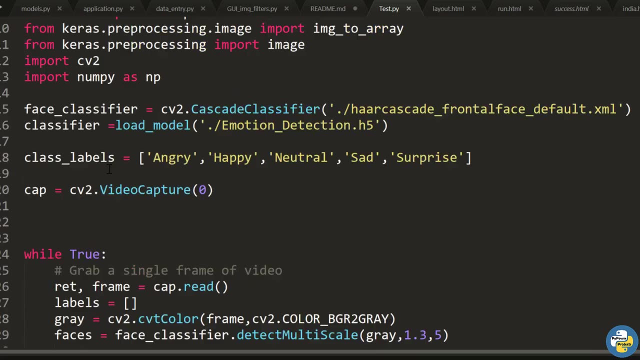 the program. if you press the Q key on the keyboard, the small Q key on the keyboard, then the loop will terminate and you will be exited from the code. and finally, the releasing task and destroying the other windows open in the project. So this way we are able to detect the emotion in a very simple way. 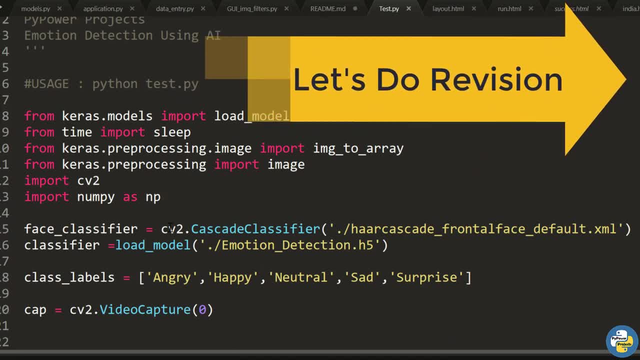 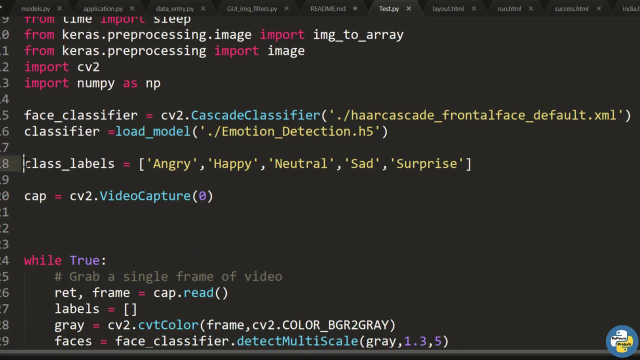 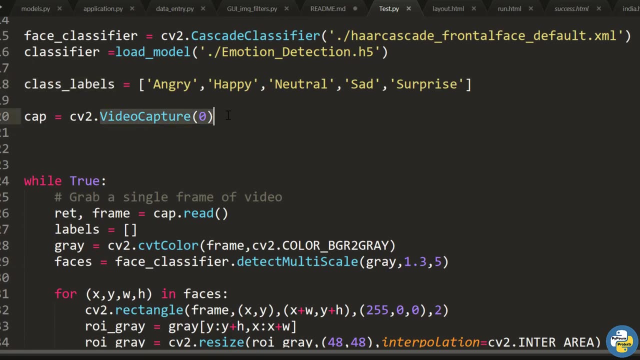 So let's revise what we have done. first of all, we have loaded the classifier- face classifier- in the emotion model By these two lines. after that, we have set the class labels which will be used for labeling the emotion. Now we are capturing the video frame after that. first of all, we have detected the face. 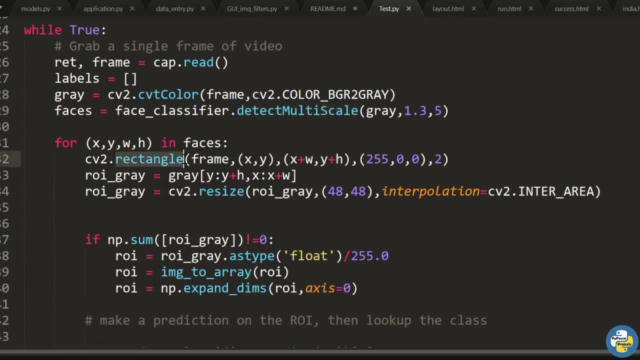 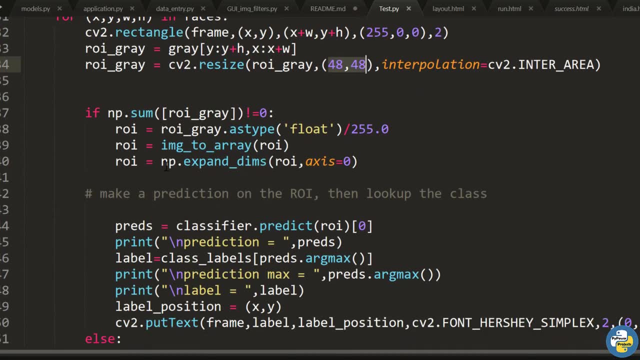 from the input image and drawn a rectangle on them by cv2.rectangle method. after that we have resized it to 48x48 for proper prediction. after that we have converted the image to array and it will be passed to this method. So let's run the classifierpredict, which will return the probabilities of each and. 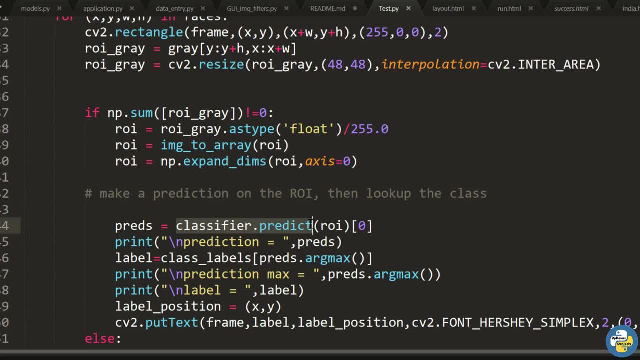 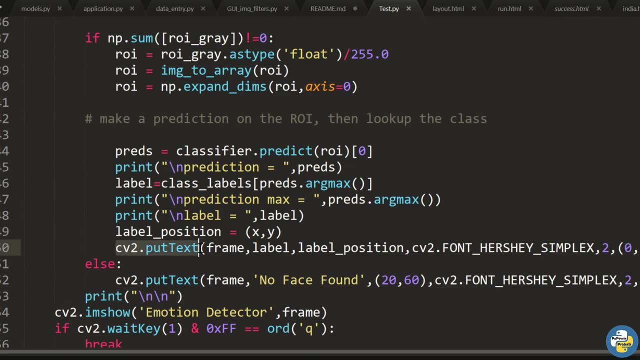 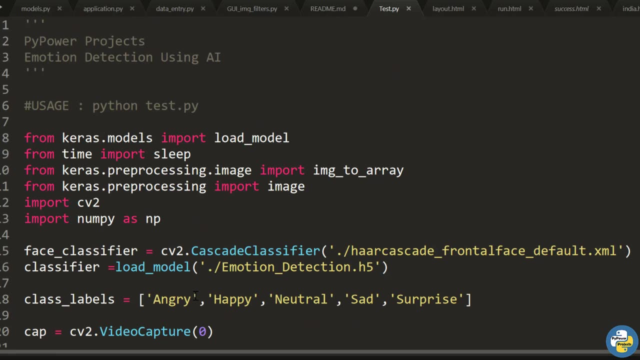 every class and we will select the class label which has the maximum probability by this function, readsargmix. and finally, we will put the text on the image for showing that. So that's it: you can run this code and you can explore the data set. you can explore the. 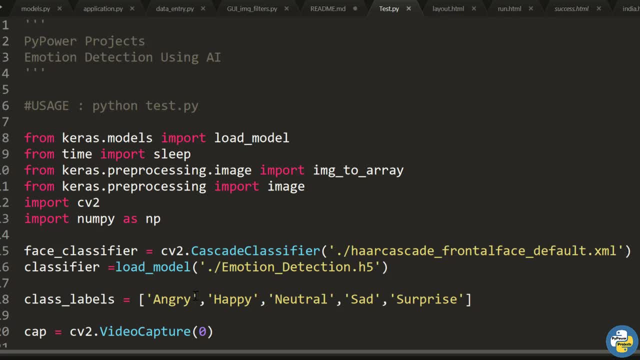 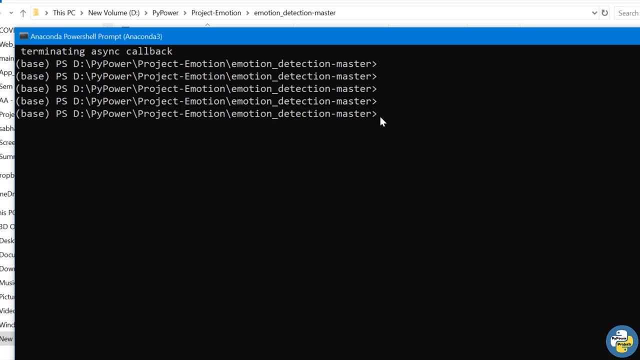 various labels and other architectures for better training and all that. So now For that you have to open the anaconda prompt and in that you have to go to the directory where the source file is kept, and after that we will use the testpy file to execute this. 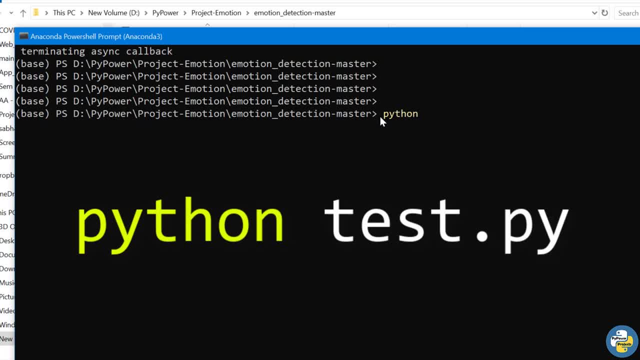 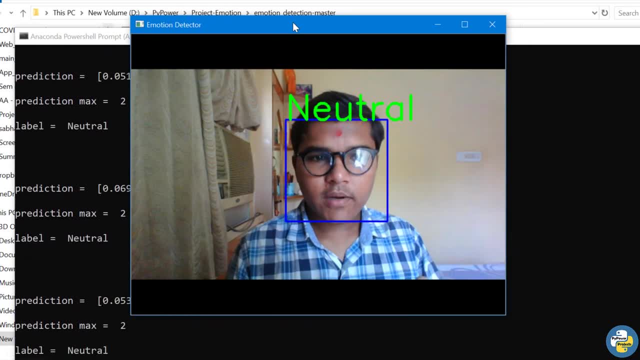 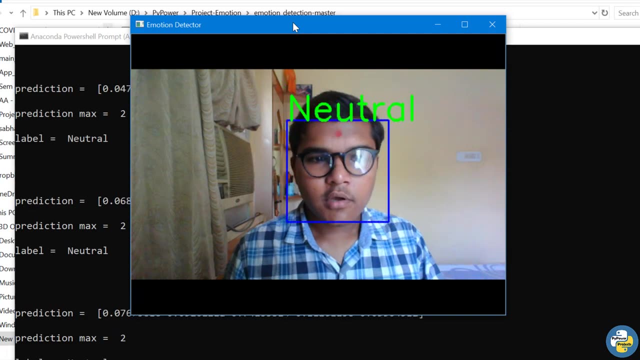 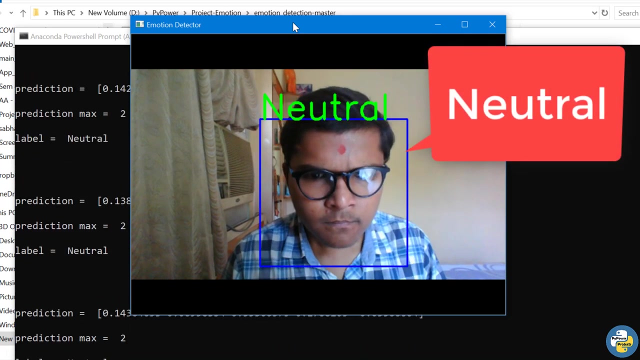 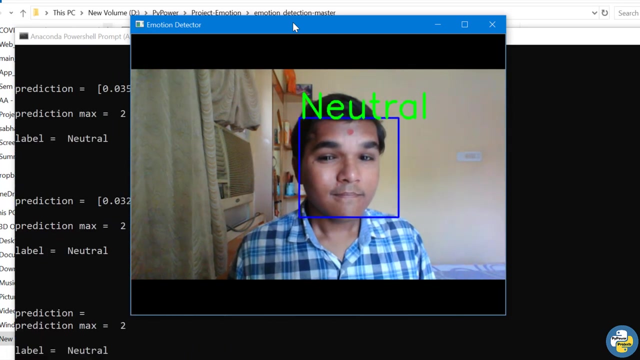 emotion detection. So you have to write python, testpy. So here you can see that in this window we are able to see the output and also the detected emotion printed above the face box. So here You can see that, based upon the emotion, the label is changing.